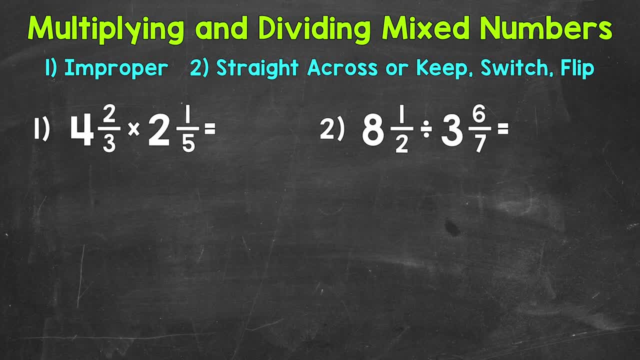 Now the first thing that we want to do here is to convert these mixed numbers to improper fractions. We do that by multiplying and then adding. Let's convert four and two-thirds to an improper fraction. So we start at the bottom and work our way to the top. 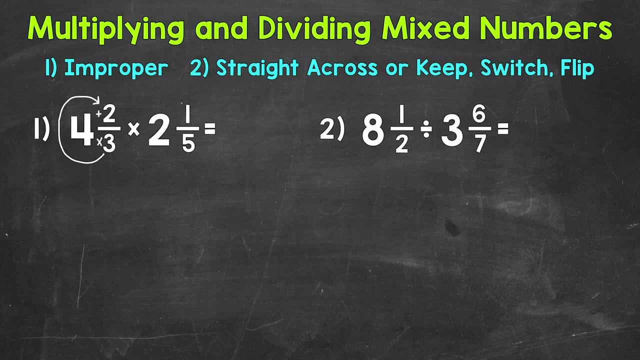 and again we multiply and then add. So 3 times 4 is 12 plus 2 is 14.. 14 is our numerator. We keep the denominator of 3 the same, So 14-thirds is four and two-thirds, and we converted. 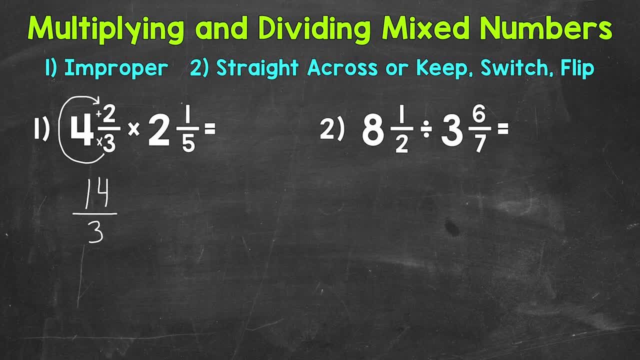 it to that improper fraction. Let's bring our multiplication sign down and then convert two and one-fifth to an improper fraction. So we multiply and then add: 5 times 2 is 10 plus 1 is 11.. So 11 is our numerator and then keep our denominator. 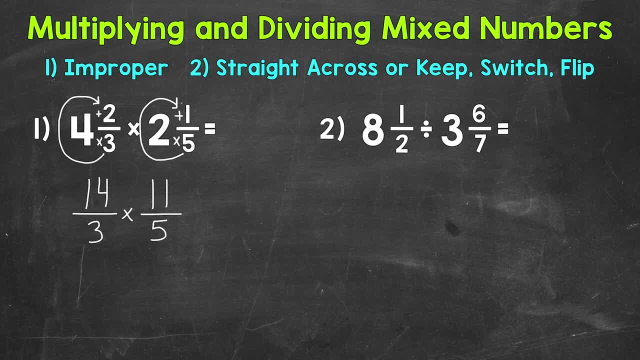 We convert these into improper fractions by adding a denominator of 5, the same Now. the reason we convert these to improper fractions is to have a numerator, a top number, and then a denominator, a bottom number. Now we can multiply straight across. So 14 times 11, that gives us 154.. 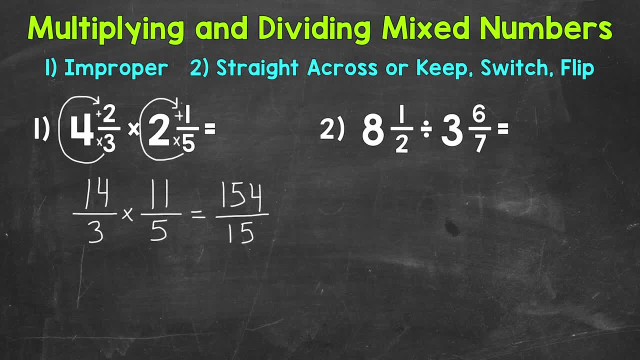 3 times 5 is 15.. So we get 154-fifteenths, or 154 over 15.. That's an improper fraction, so we want to convert this back to a mixed number for our final answer. So we do that by dividing 154 by 15.. 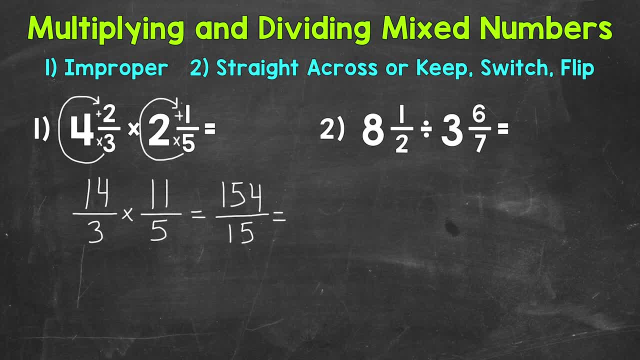 How many whole groups of 15 can we pull out of 154?? Well, 10.. That gets us to 150.. Now, we did not hit 154 exactly, We had a remainder of 4, so that's our numerator, and then keep our denominator of 15 the same. 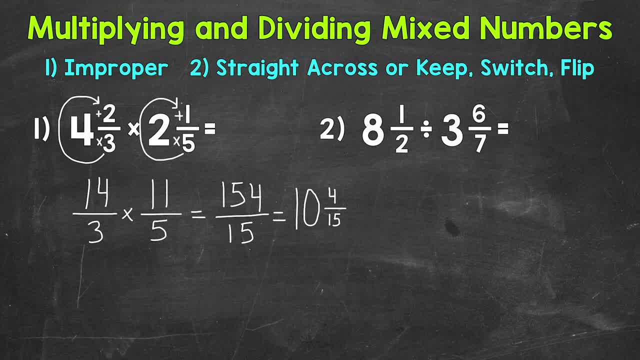 Always look to see if you can simplify the fractional part of a mixed number- 4- 15ths. well, the greatest common factor between 4 and 15 here is 1, so this is simplified and done: 10 and 4- 15ths. 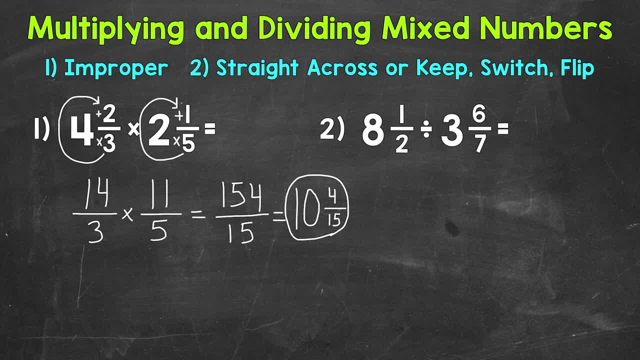 So, to recap, convert to improper fractions and then we can multiply straight across. Okay, Let's move on to number 2, where we have 8 and a half divided by 3 and 6 7ths. So we need to convert these to improper fractions. 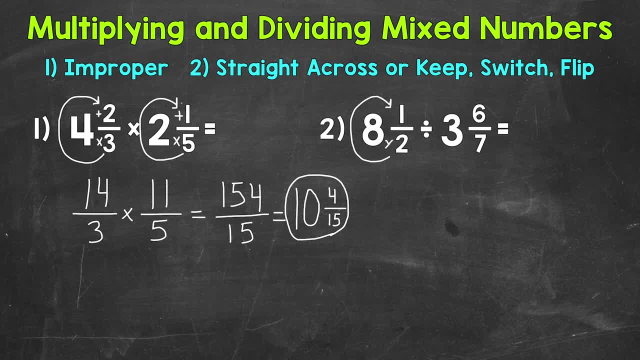 Start at the bottom, work our way to the top, multiply and then add. So 2 times 8,, that's 16, plus 1 is 17.. Keep our denominator of 2 the same. Bring our division sign down here. 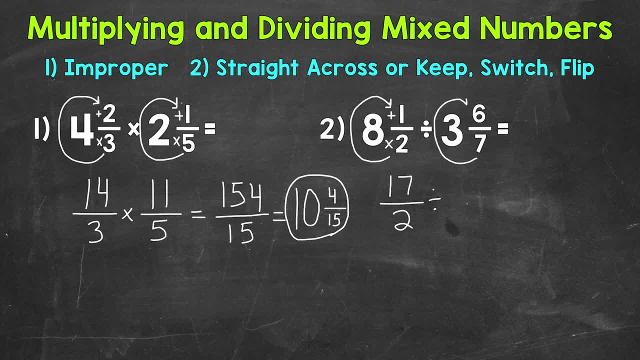 And then 3 and 6, 7ths. So multiply and then add 7 times 3 is 21, plus 6 is 27.. So that's our numerator. Keep our denominator of 7 the same. So now we have numerators and denominators only, and we can go through our dividing fractions. 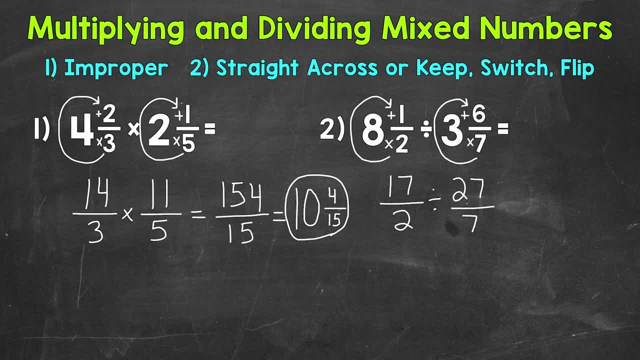 steps: Keep, switch, flip. So we always keep our first fraction. So let's rewrite this problem using those steps: Keep 17 over 2. Switch division to multiplication- The opposite of division here. So switch to multiplication. And since we switched to the opposite of division, we're going to flip our second fraction. 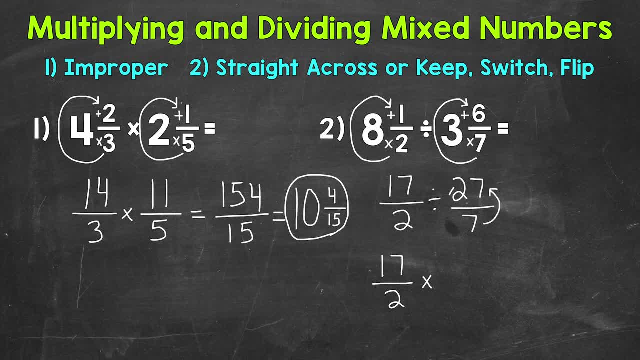 Meaning the 7 is going to be our numerator And the 27 is going to be our denominator And the 27 is going to be our denominator. This is called the reciprocal. So the 7 is now the numerator and the 27 is now the denominator. 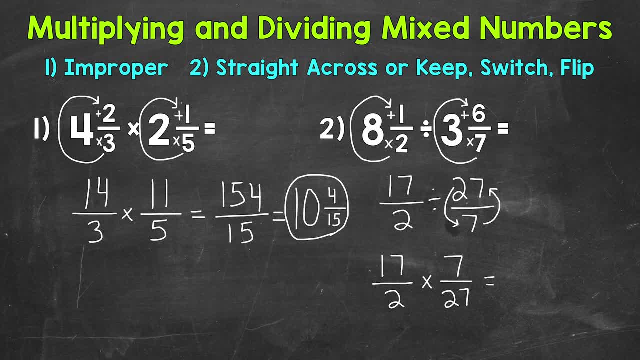 Now we can multiply straight across, So 17 times 7, and then 2 times 27.. Now just a side note here. If you need to solve something to the side, for example 17 times 7,, you can come to the. 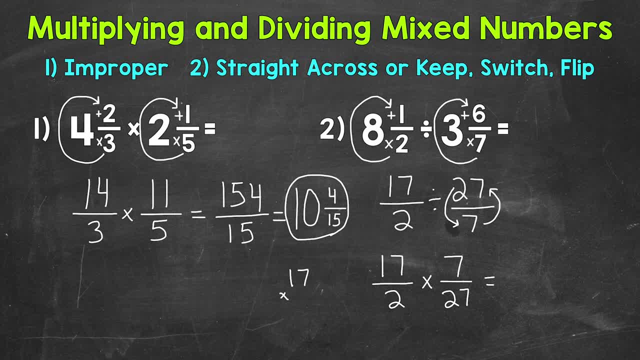 side and let's multiply here 17 times 7.. Well, 7 times 7 is 49.. 7 times 1 is 7, plus 4 is 11.. So 119.. It's okay to come to the side to solve things if need be.